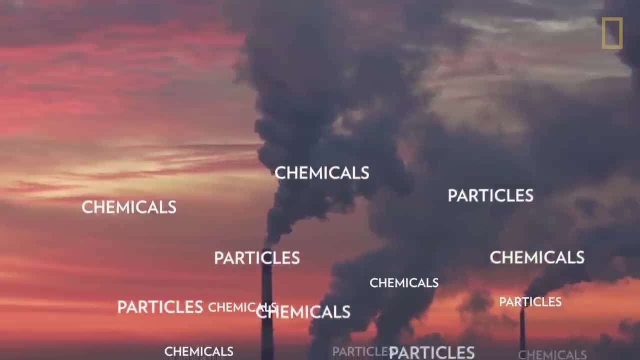 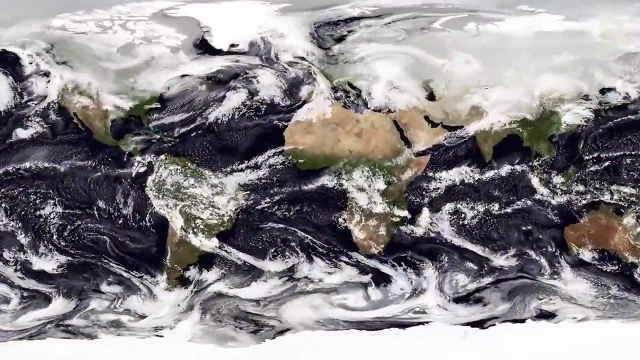 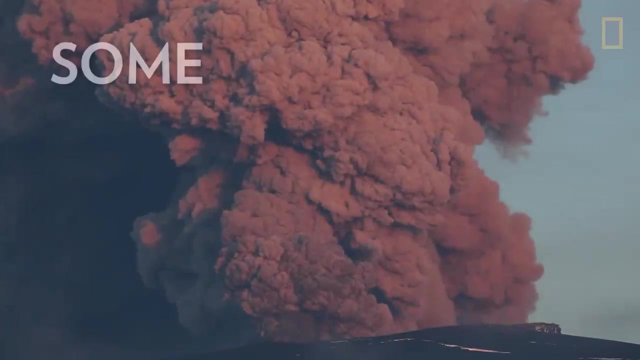 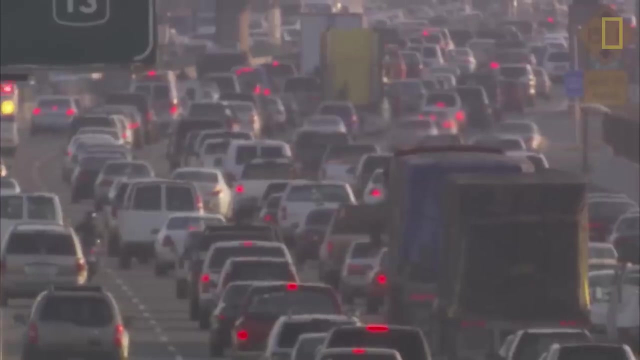 Air pollution consists of chemicals or particles in the atmosphere that pose serious health and environmental threats. But what causes air pollution and what does it mean for our planet? Some air pollution comes from natural sources like volcanic eruptions, wildfires or allergens, But most air pollution results from human activities, such as energy use and agriculture. 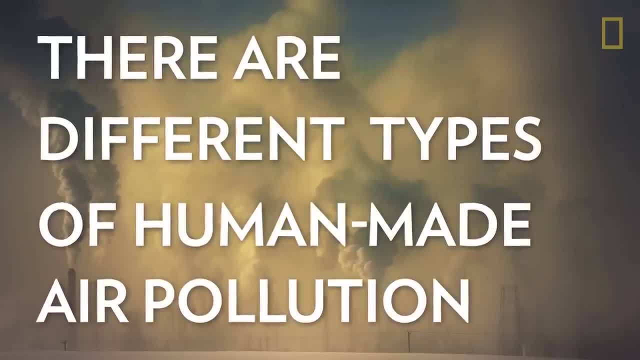 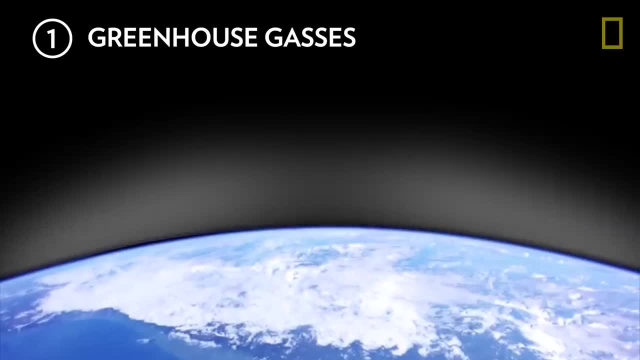 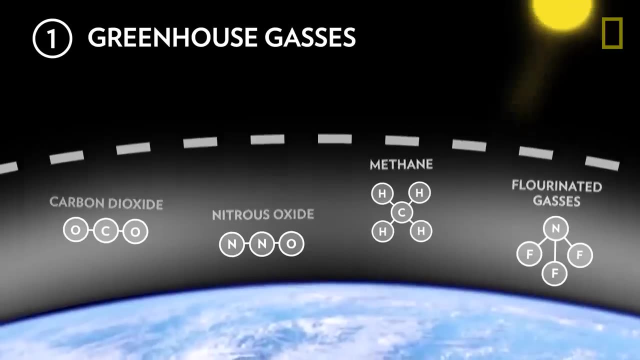 There are different types of human-made air pollution. When we burn fossil fuels to produce energy, they release greenhouse gases into the air. These emissions, such as carbon dioxide, methane, nitrous oxide and fluorinated gases, trap heat from the sun in Earth's atmosphere, leading to a rise in global temperature. 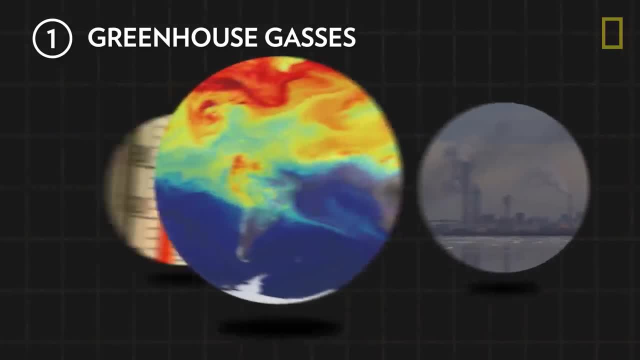 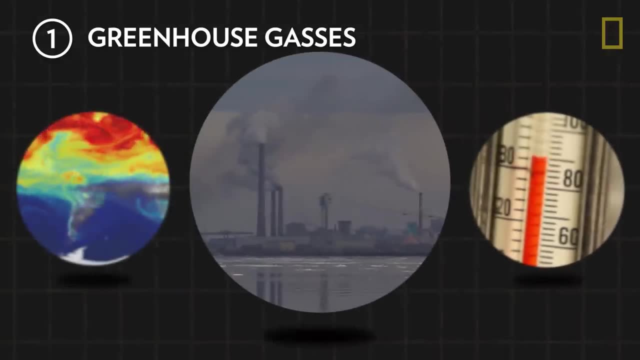 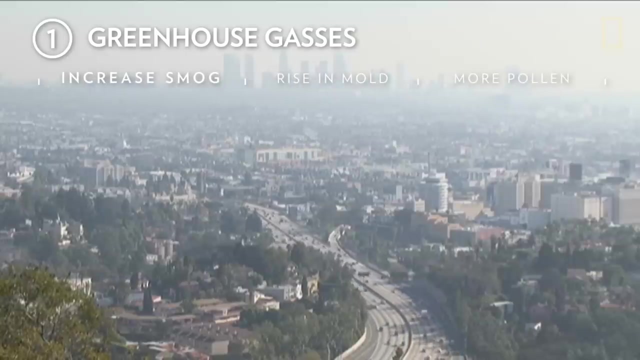 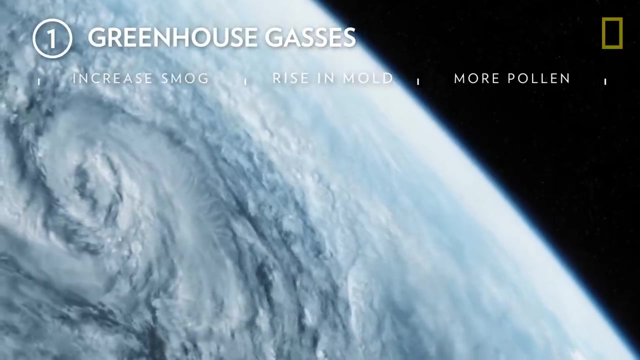 This creates a cycle where air pollution contributes to climate change and climate change creates higher temperatures. In turn, higher temperatures intensify some types of air pollution. For example, climate change increases smog because it forms, in the presence of high heat and increased levels of ultraviolet radiation, More frequent extreme weather. 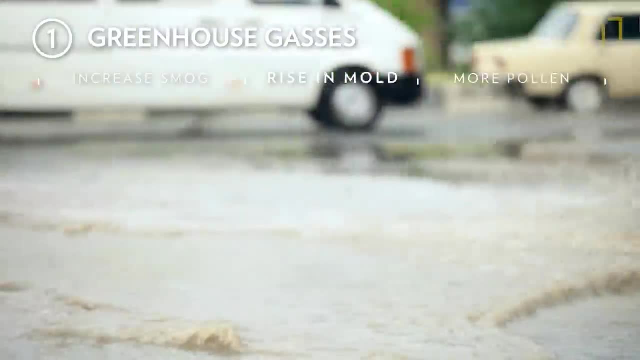 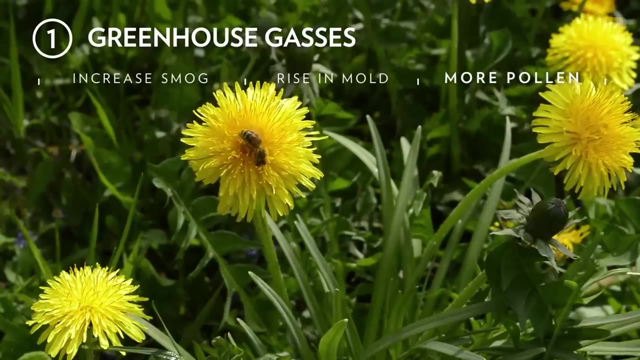 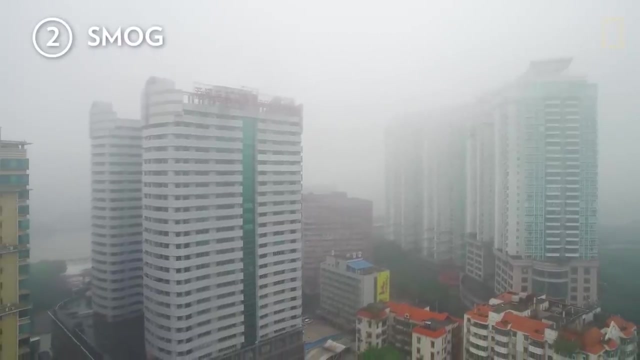 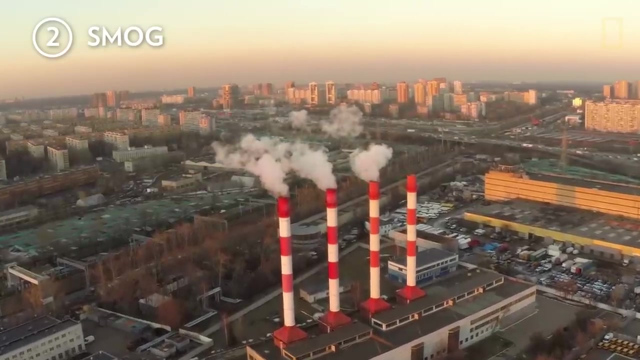 such as flooding, contributes to damp conditions and heat, And therefore to a rise in mold. Warmer weather also leads to longer pollen seasons and therefore more pollen production. Smog is a type of air pollution that reduces visibility and has serious health effects. Smog can be divided into two categories: sulfurous and. 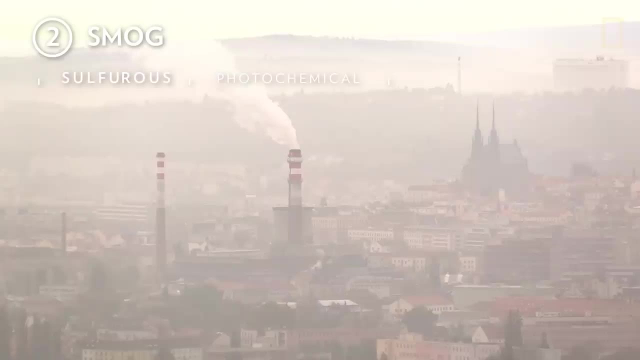 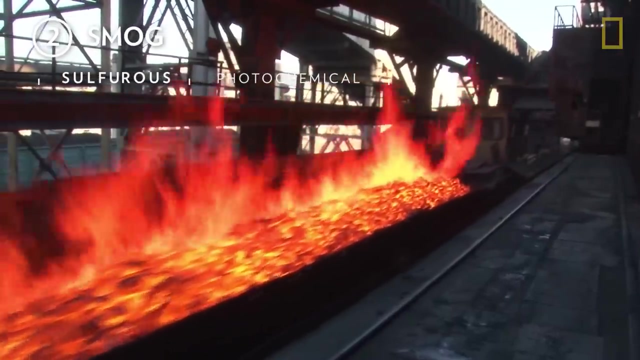 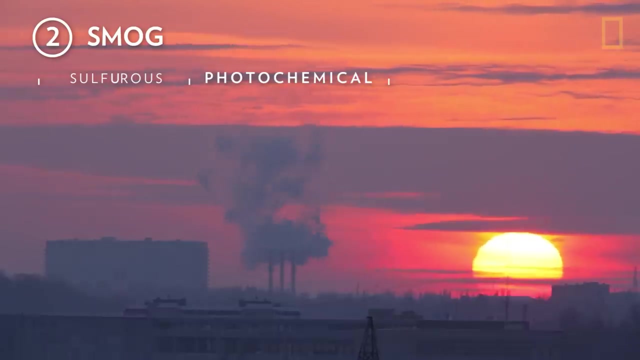 photochemical Sulfurous smog is made up of chemical compounds called sulfur oxides. It occurs when burning sulfur-bearing fossil fuels such as coal. Photochemical smog, also called ground-level ozone, is a result of the reaction between sunlight, nitrogen oxides and volatile organic. 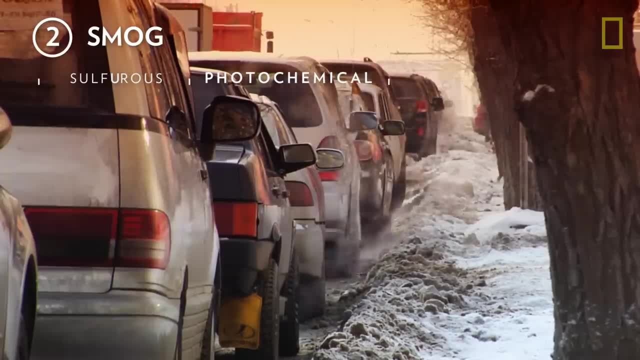 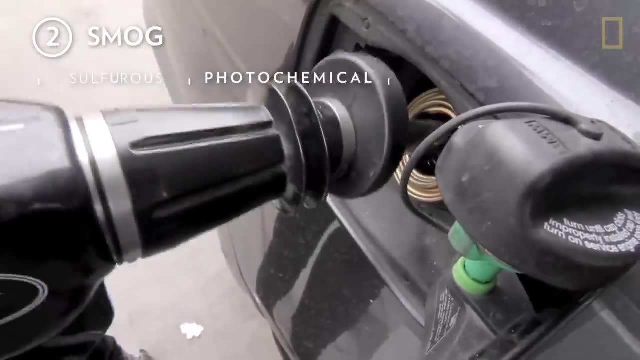 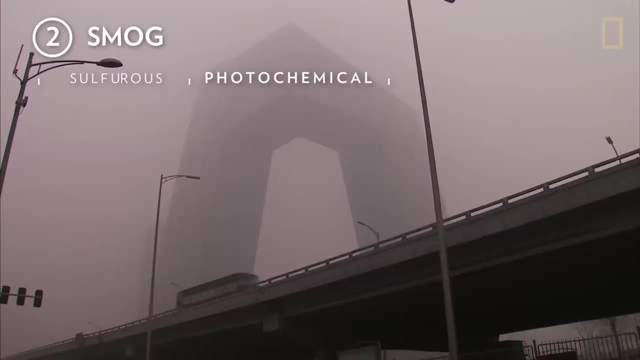 compounds. Nitrogen oxides come from car exhaust, coal, power plants and factory emissions. Volatile organic compounds are released from gasoline, paints and many cleaning solvents. Smog not only creates a brown haze that reduces visibility, but also harms plants, irritates the eyes.